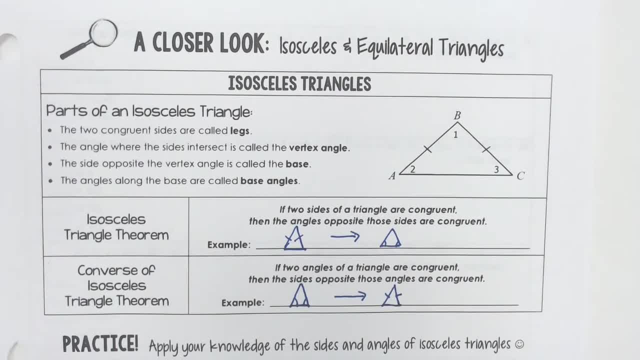 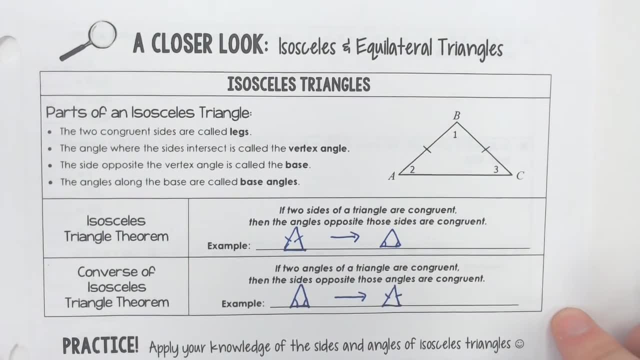 would be equal. So that's all that those mean and that's what I described at the beginning as well. So we're going to do a few practice problems with this. It's not hard to do. It just is more of a figure out what angles are equal and what sides are going to be equal, type of thing. 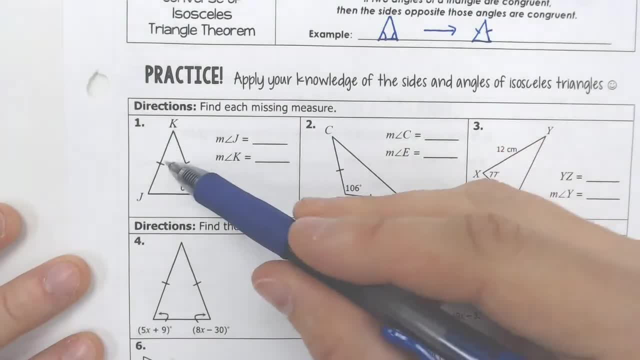 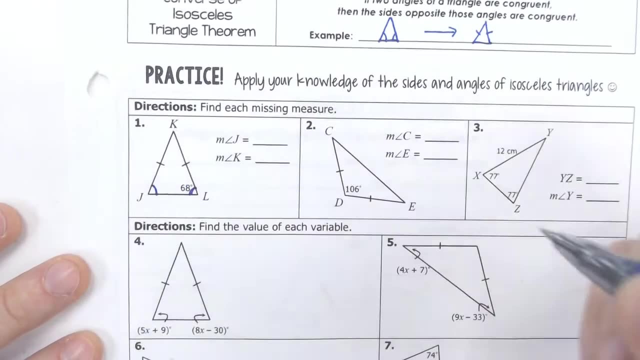 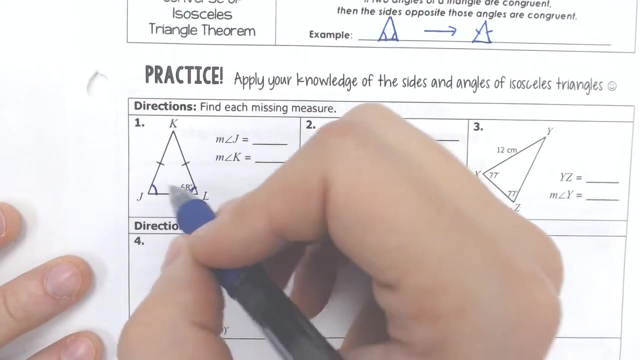 So number one: we have these two sides right here that are equal. That would tell me that angle L and angle J are going to be congruent as well for this isosceles triangle. So, on this isosceles triangle, we have these two sides that are equal and we have these two angles that are equal. That would tell me that. 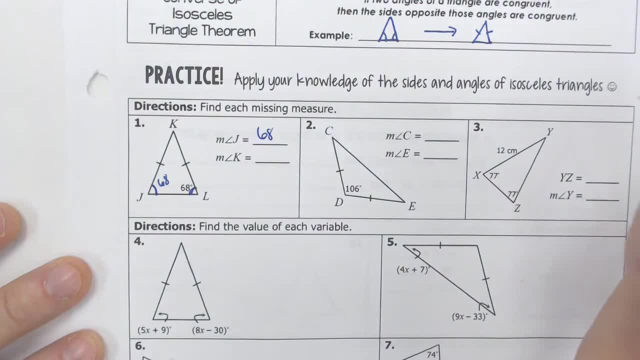 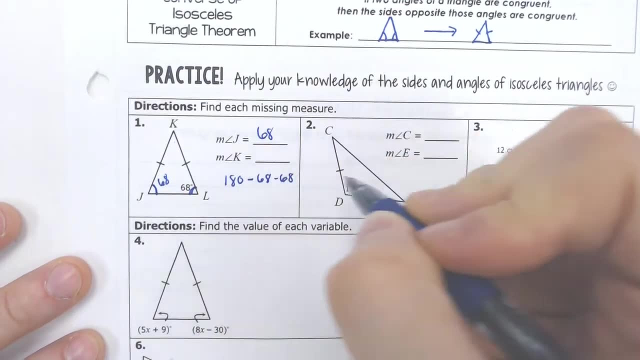 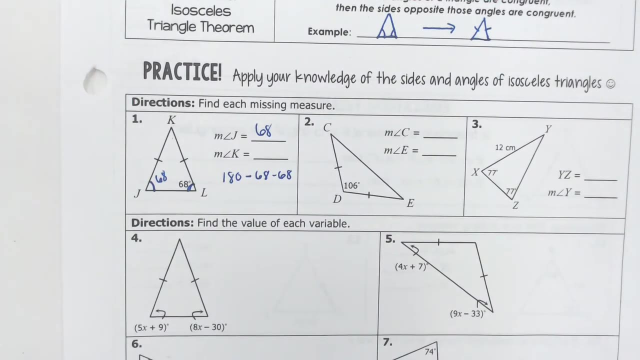 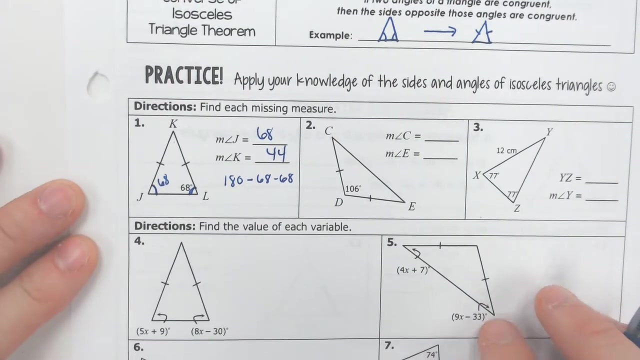 angle J is 68 degrees. Now, in order to find out angle K, all we have to do is 180 minus both of those 68s and we would get our answer. So we're going to do a few practice problems with this. So 180 minus 68 and minus another 68 is 44 degrees. For number two, we have a very similar 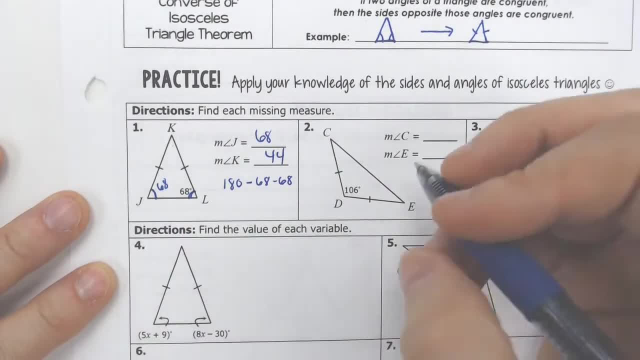 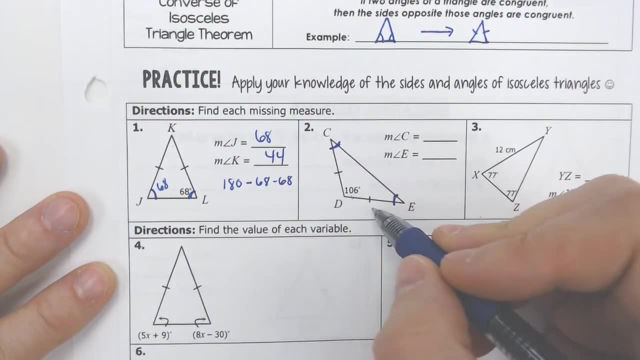 thing. but instead of being told what one of the equal angles are, we know that these two angles are equal because the 106 is in between the two sides that are congruent. So C and E, those angles are going to be equal. So we're going to do a few practice problems with this. So 180 minus 68 and 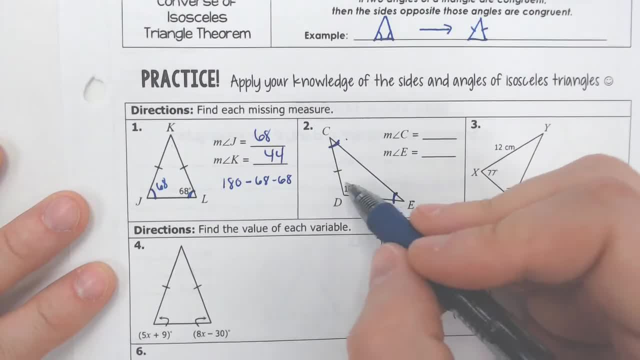 whatever we find for one, we're going to have for the other, And this 106 is the part that we're given. So what we can do is we can take 180 and we can set it up to those two equal parts that we could call X. We can call them both X. So 180 would equal X plus X and the 106.. So we would have. 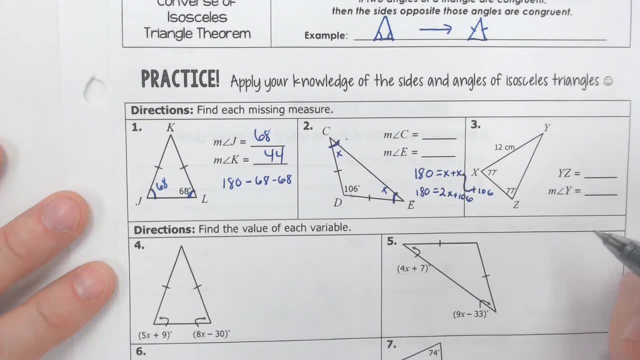 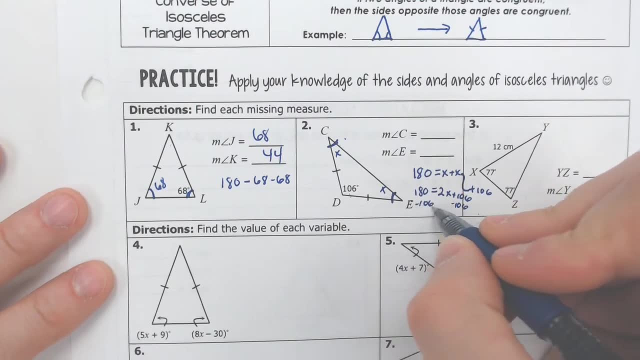 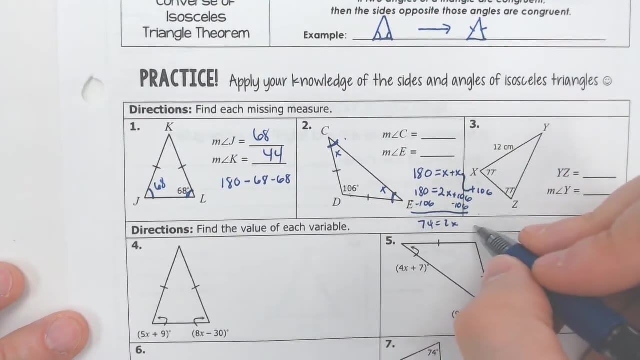 180 is equal to essentially 2X plus 106. So we would have: 180 is equal to essentially 2X plus 106.. Subtract 106 from 180 and you would end up with a. 74 is equal to 2X, And when you divide 74 by 2, 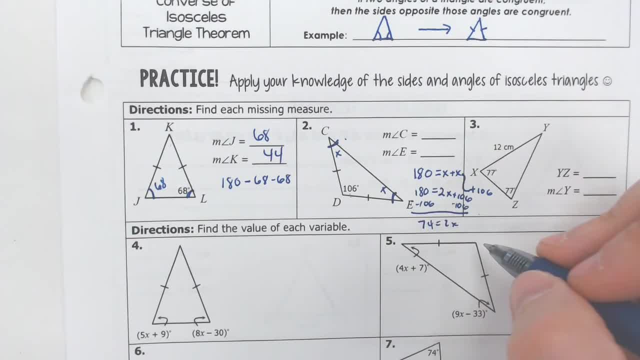 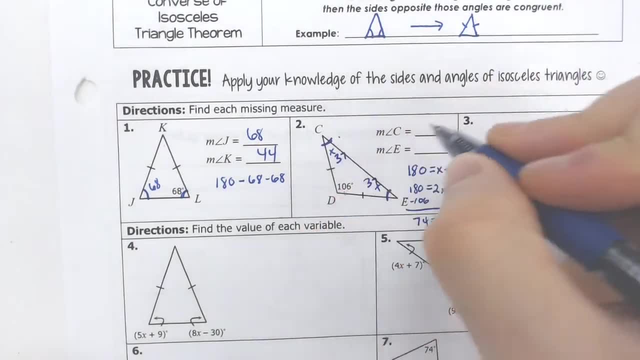 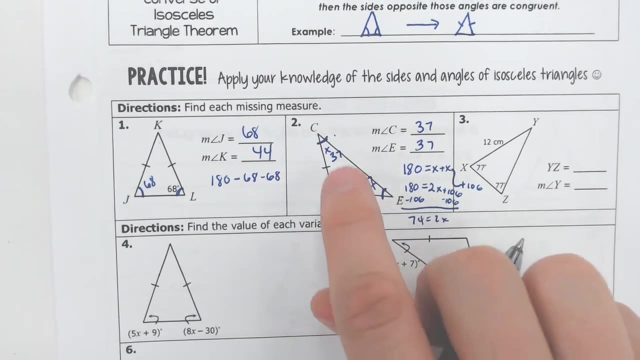 you end up with, I think, 37.. 74 divided by 2 is 37. So that means that both of these angles are 37.. Now I showed you an actual, like more equation-y way to do this, But in reality, if it's only giving you numbers and not a lot of Xs and stuff, what you can do is you can. 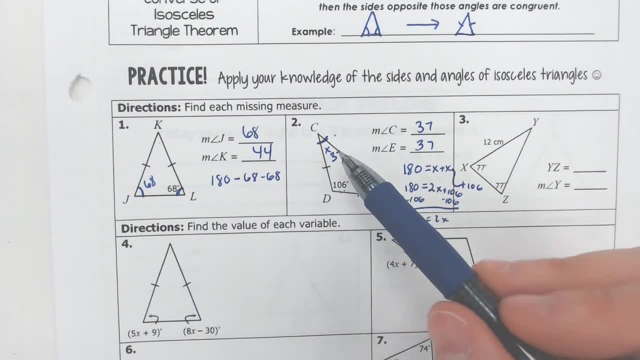 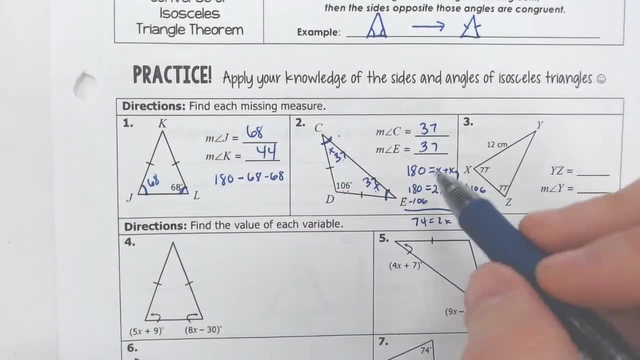 realize. well, wait a minute, if this is 106, then I know that the remaining part of the triangle would have to be split evenly. So I could take the 106 away from 180, which we did, and then split it evenly means divide it by 2, which we did as well. We took 106 away from 180, got 74, we divided by 2, and that's. 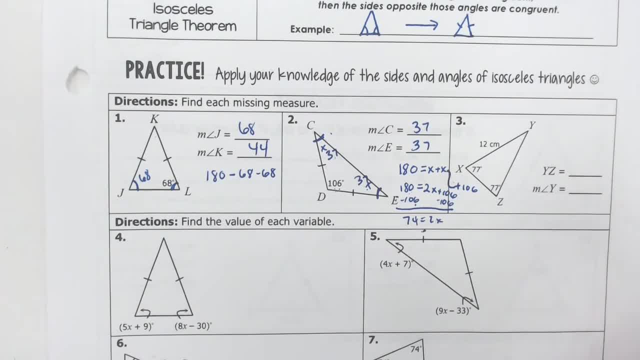 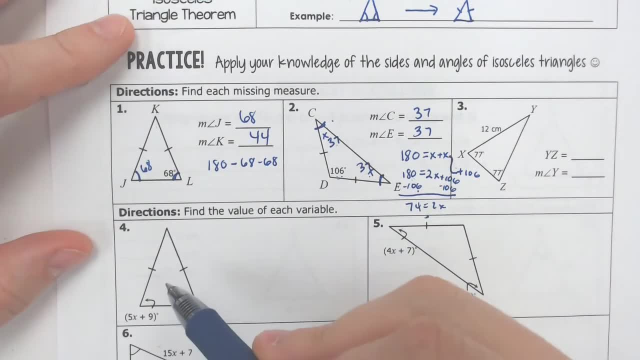 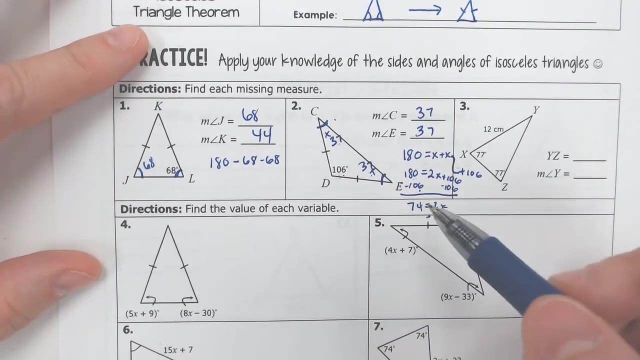 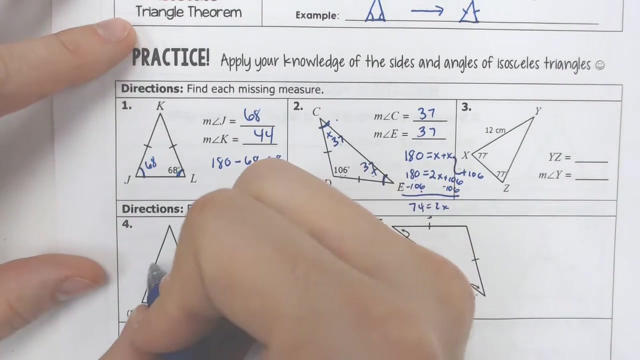 how we got the 37s. So, moving on, we're going to deal with a little bit more of a scenario where we have equations. So in the equation, sometimes you'll be equaling them to each other and other times you will be adding them to equal 180.. It really depends on the scenario. You have to be very close into the sides. 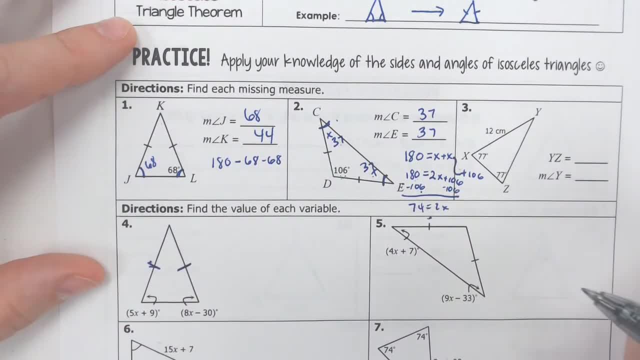 that are equal. and on number 4 these two sides are equal, which means these two angles down here would be equal, That 5X plus 9 is equal to 180. So in this case, even though they're angles, we're not going to set it equal to 180, we're going to set them. 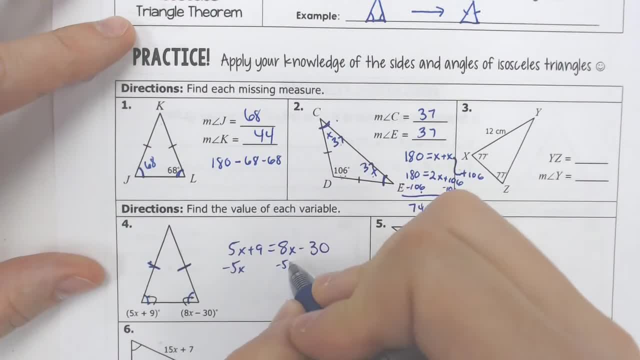 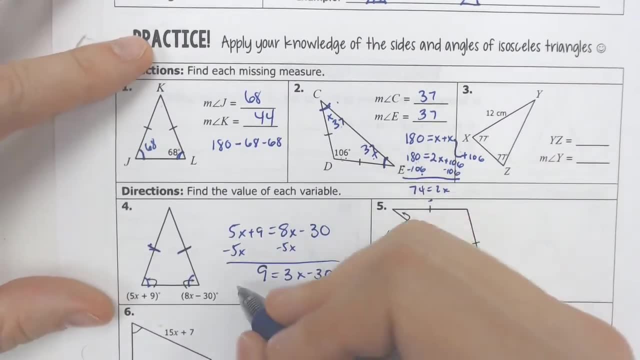 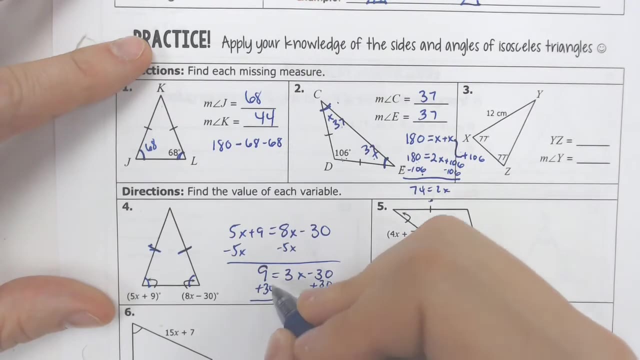 equal to each other. So I'm going to subtract 5X, get 9 equals 3X minus 30, and then I'm going to have to add 30 to the other side to get the 3X. by itself We end up with 3X is equal to 39, and when we divide, 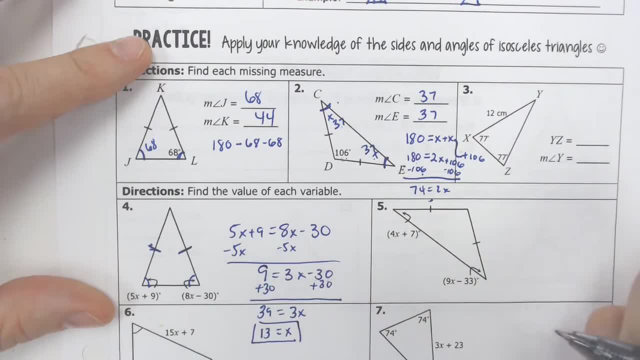 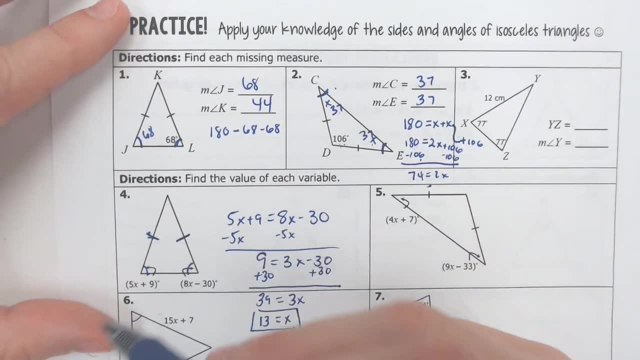 39, we get 9 equals 3X minus 30. So again in this problem it was more of a matter of hmm, even though they're angles, I know they're equal to each other. so it's the first time in a while we haven't been adding things to equal 180. 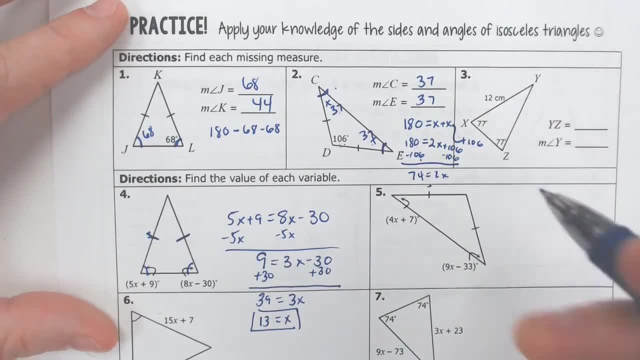 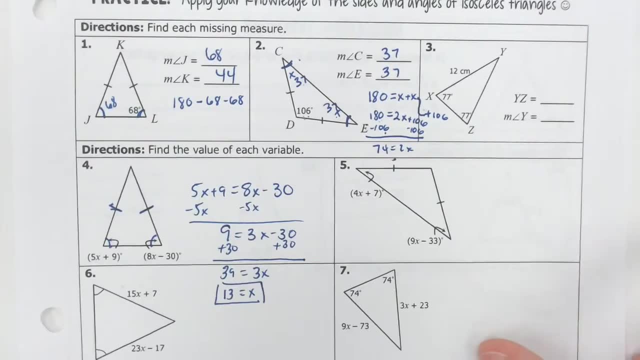 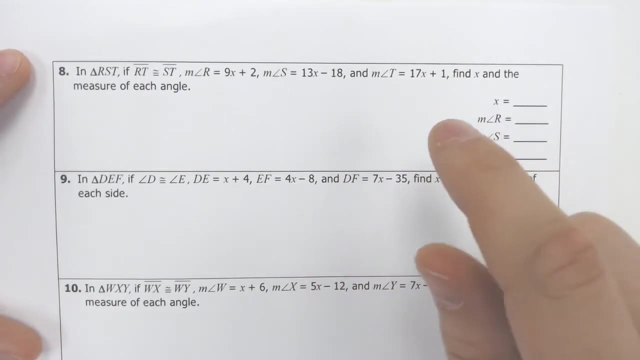 they equal each other, and that's the equation I would have to solve. Moving on to the back of our sheet, you'll notice something that is slightly annoying, and that is that these don't give you the same value as the other side. They don't give you a triangle, so you need to draw the triangle so it tells you this is triangle RST. 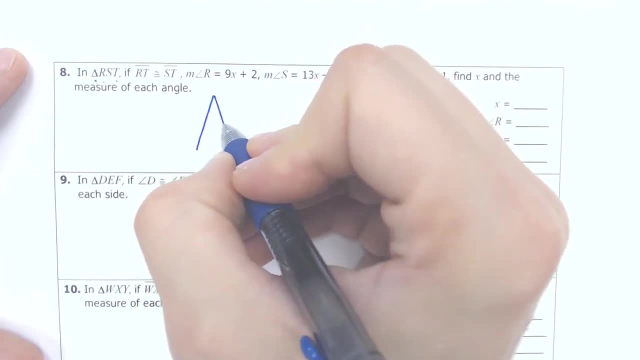 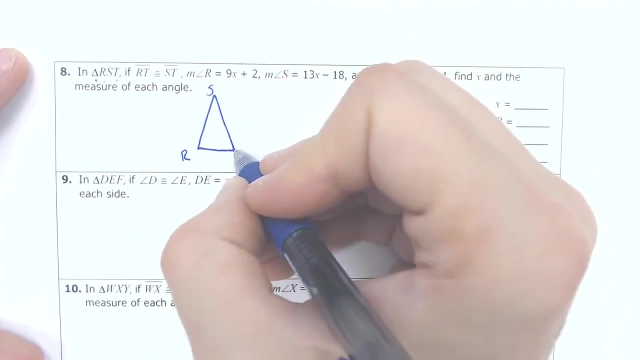 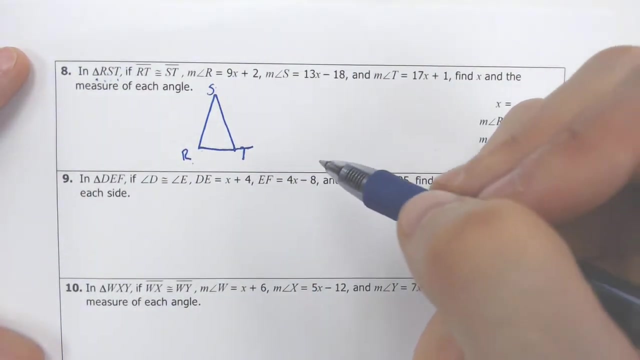 So I'm going to draw a triangle RST. It does not really matter where you start it, but I like to start normally in the bottom left hand corner, just because it's how I write English as well. So I have RST. I've labeled my points from here. 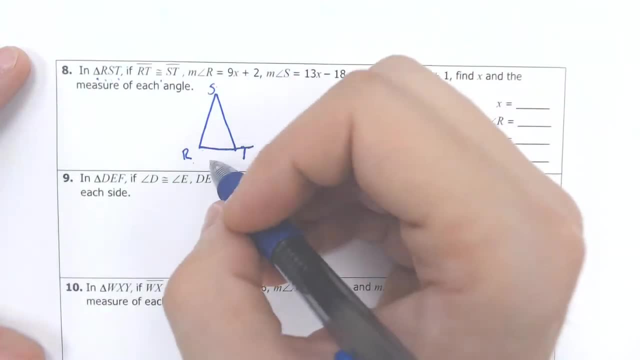 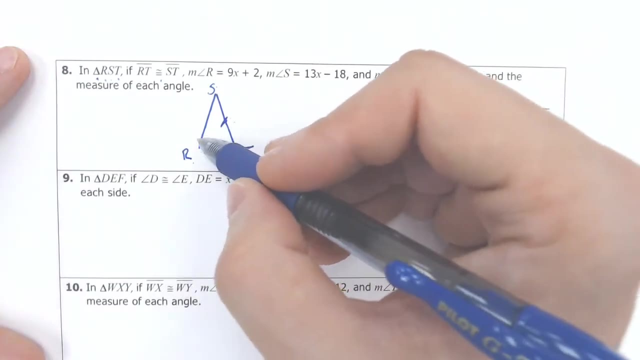 It tells us that RT is equal to ST. You know you may notice that I didn't really draw it to scale, so you may choose at this point to redraw it If these don't look like they're equal. I made it look like RS and ST were equal, so you may choose to redraw it. 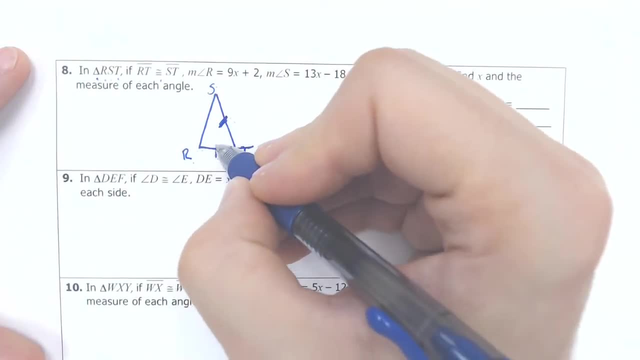 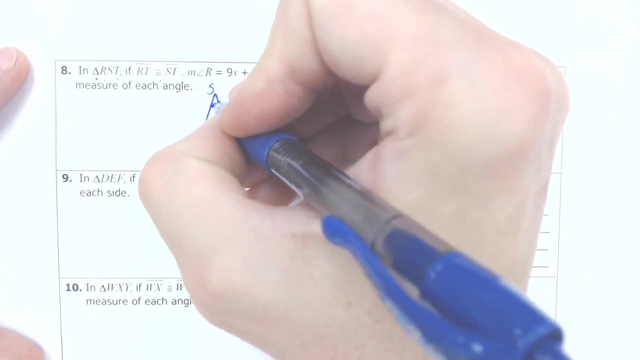 It's up to you. I know that these are equal. I was told they're equal. I'm just going to let it be known that those two are the equal sides, which means these would have to be the equal angles, because the angles that are equal are the ones that are the base angles. 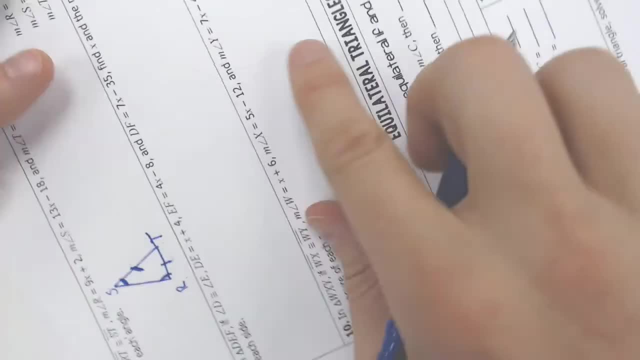 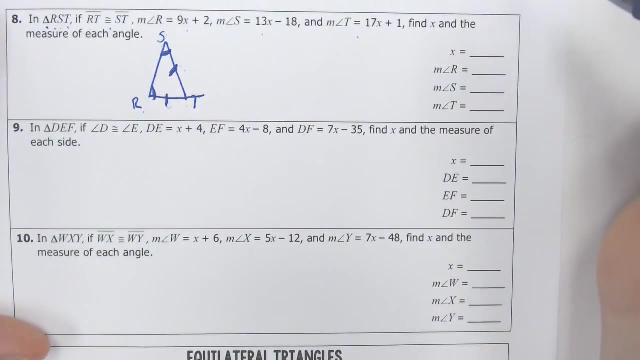 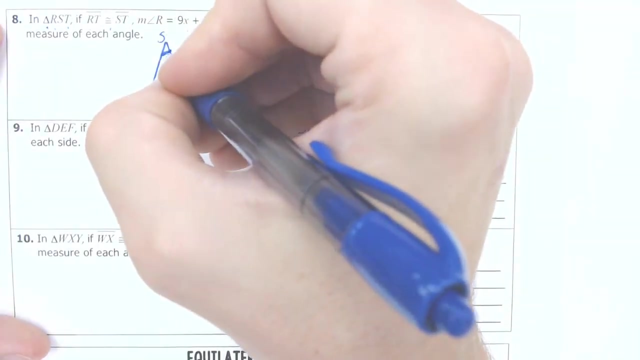 of those two. So I've set those equal to each other. and now I'm told some more information. I am told all three of the angles here. So if I'm told all three of the angles, I actually have a few different options. So I know that angle S and angle R are going to be equal to each other. 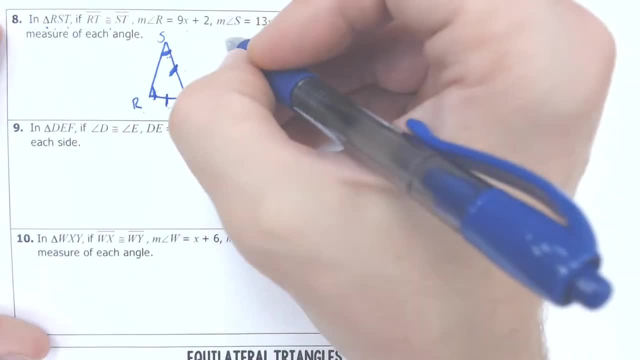 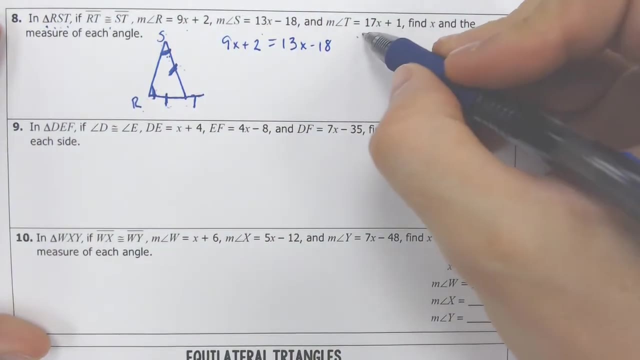 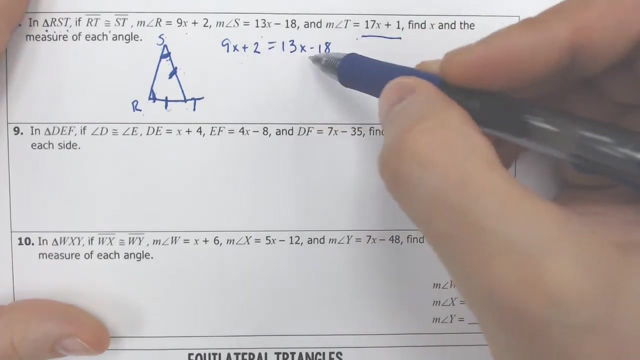 It says it right here from my hash marks, so I can literally set these equal to each other. But I was also told what angle P is. So if I know what angle T is, if I know all three angles of a triangle, instead of setting these two things equal to each other I could have just added all three of them up to equal 180. 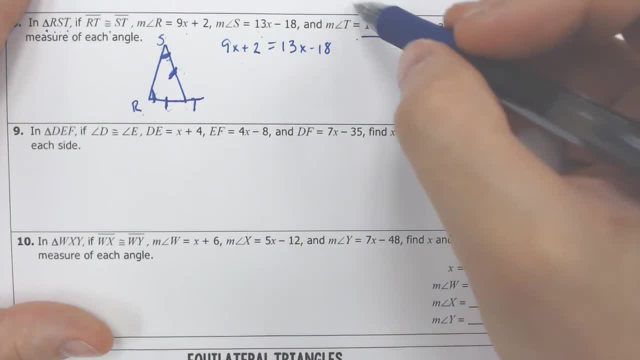 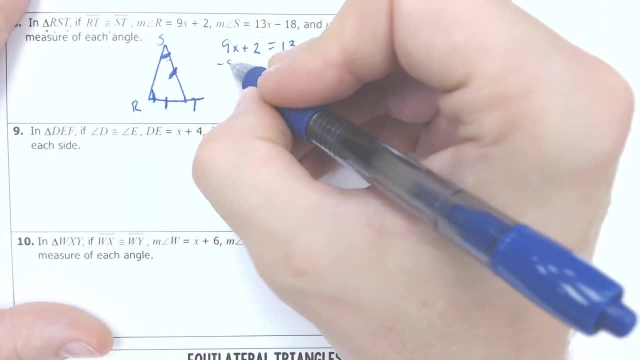 But they didn't have to give a single T, that was just a gift. So most likely you're going to have to set these two things equal to each other. So I'm going to subtract: 9x 2 would equal 4x minus 18.. 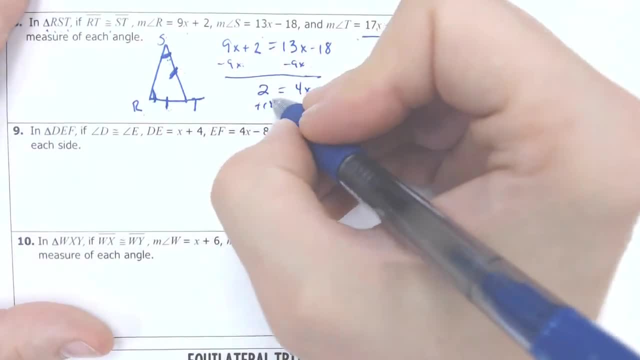 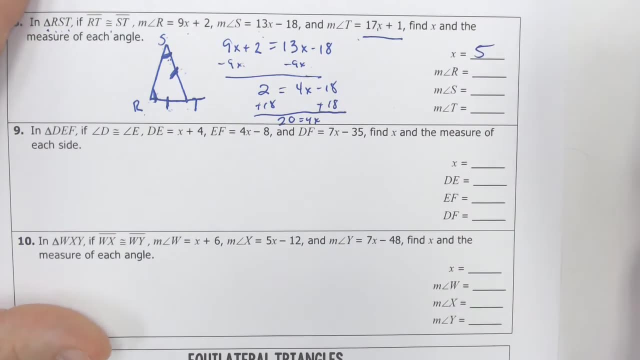 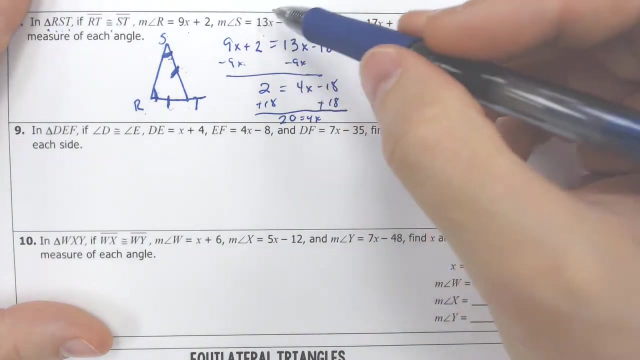 And add 18.. And add 18.. Add 18.. And add 18.. 20 is equal to 4x, And if you divide 20 by 4, you get 5 for x. And then, once you get 5, you would be expected to plug in 5 for each and every single x to find R, S and T out. 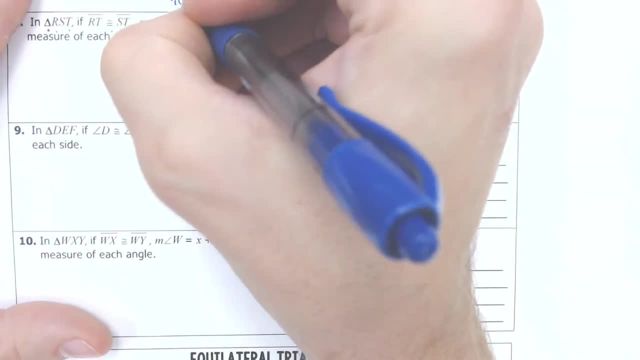 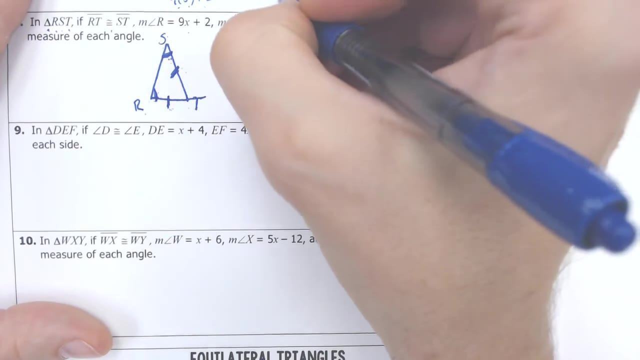 So I'm going to plug in 5 real quick. 9 times 5 plus 2 is 45.. Plus 2 is 47.. I'm going to plug in 5. minus 18.. I know that's 47 as well. How do I know it's 47? Because r is supposed to equal t. 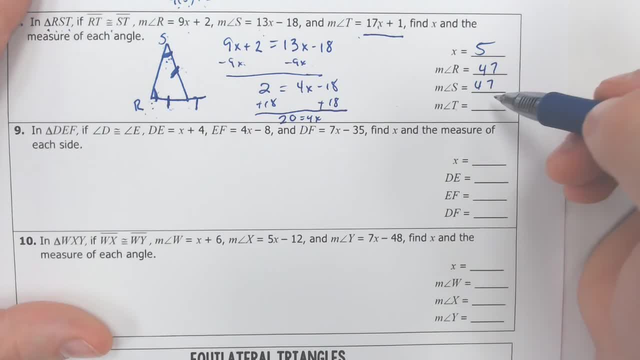 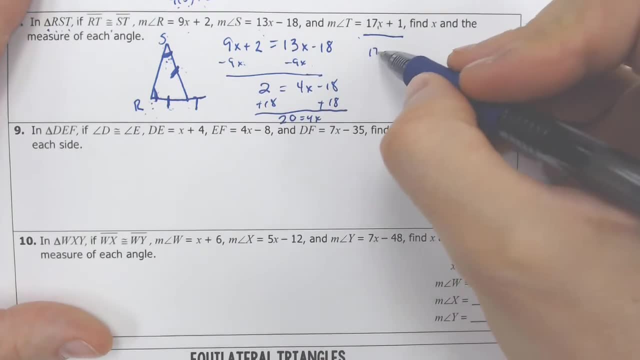 So once I knew r, I knew t as well. I said t: r is equal to s. Once I knew r, I would know s. Now I can plug in the 5 here 17 times 5 plus 1.. That one's a little harder. I'm going to use 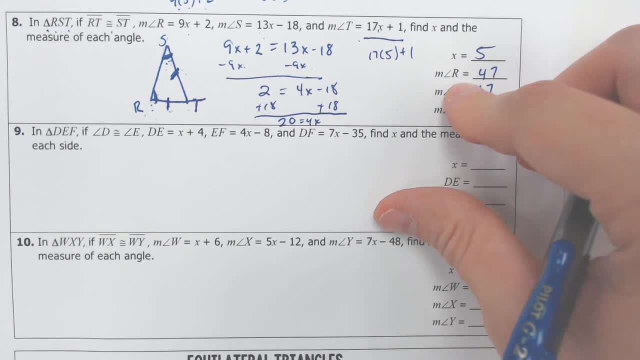 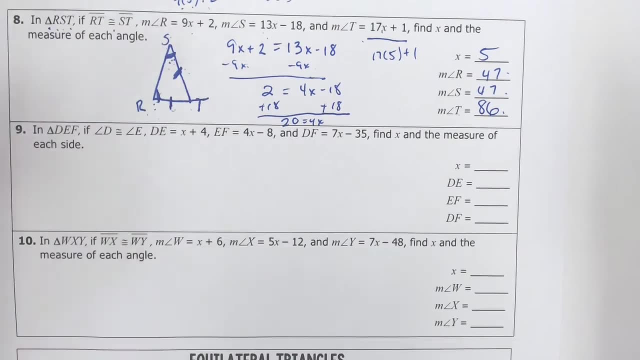 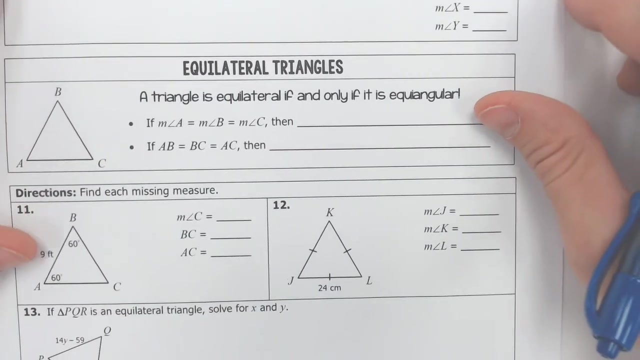 calculator: 17 times 5 equals 85 plus 1 makes 86. If I add all three together, I should get 180, because it's still a triangle. They still add to 180.. Moving all the way down to the bottom of the page, we have equilateral triangles, Equilateral. 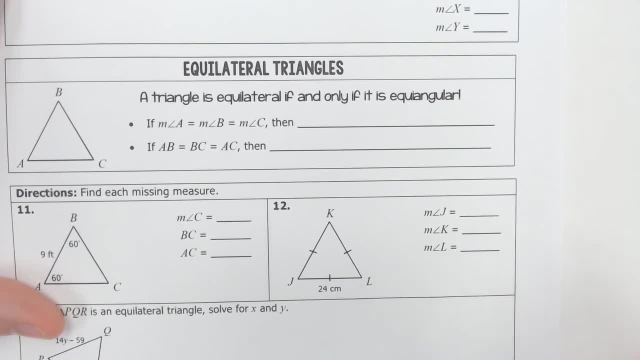 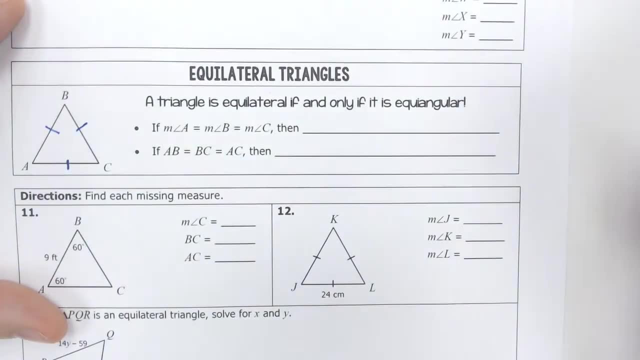 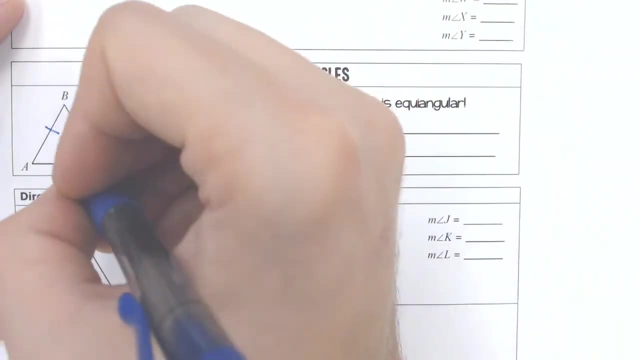 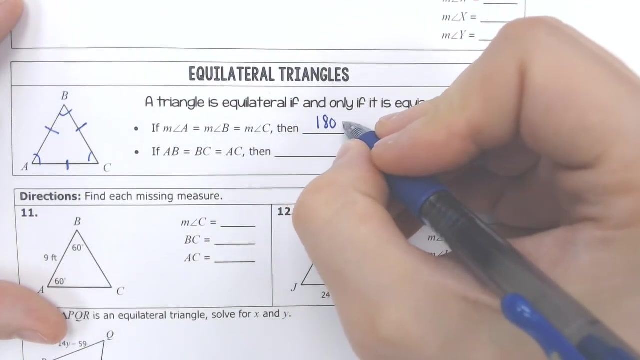 triangles are kind of how they sound. All sides are equal. So if all the sides are equal- a, b, b, c and a- c- all those sides are equal- then that would mean that all the angles are also going to be equal. And if all the angles are equal, you could take 180 and divide by 3.. 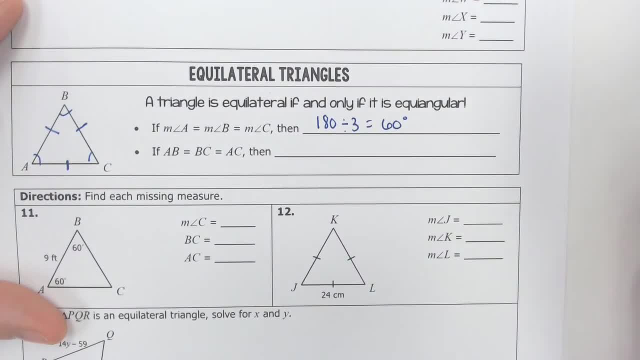 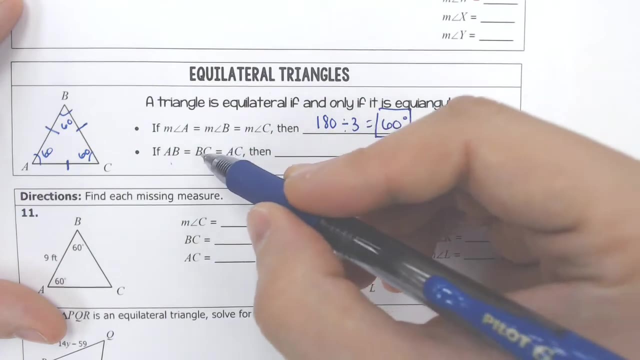 Every angle would have to be evenly divided into threes and each one would have a share of 60 degrees. Every equilateral triangle, the angles, will equal 60 degrees. And here it's saying that if a b is equal to b c and b c is equal to a c, 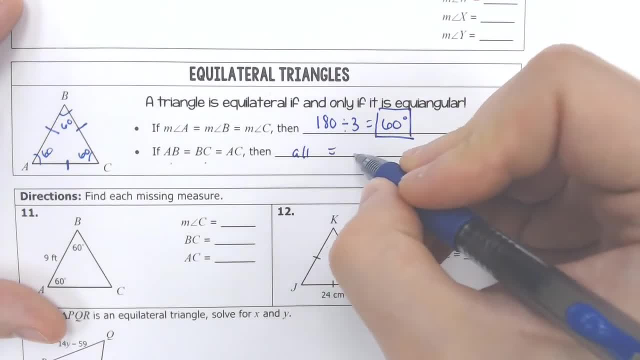 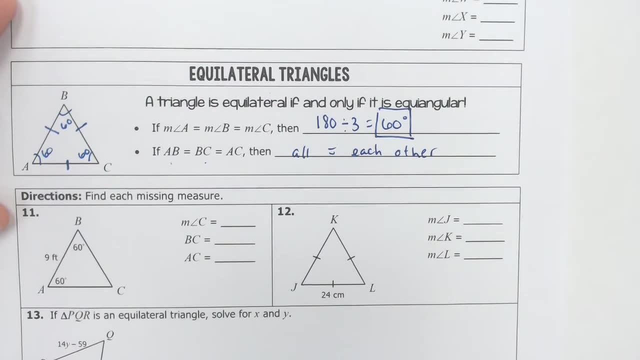 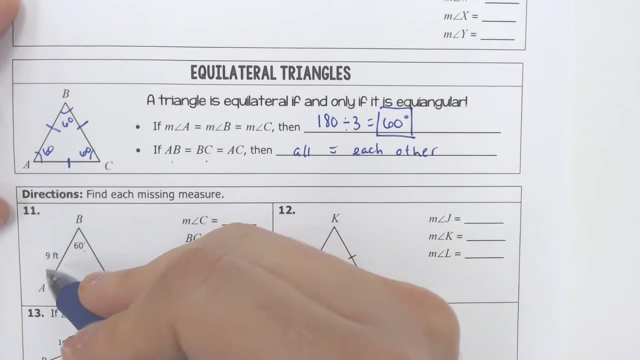 then they all equal each other. I don't know what they were even trying for that line. So in these problems they're just going to confirm in some scenarios that if these are 60, so would this be. If this is 9,, all of them would be 9.. 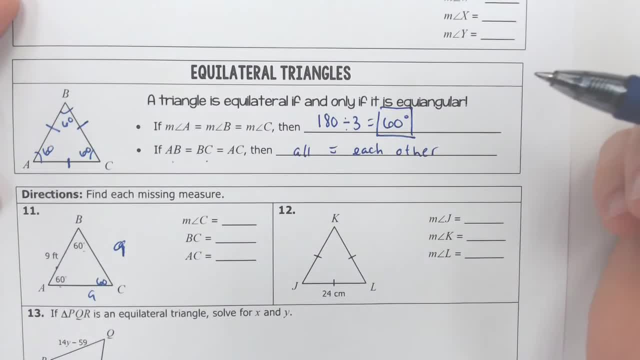 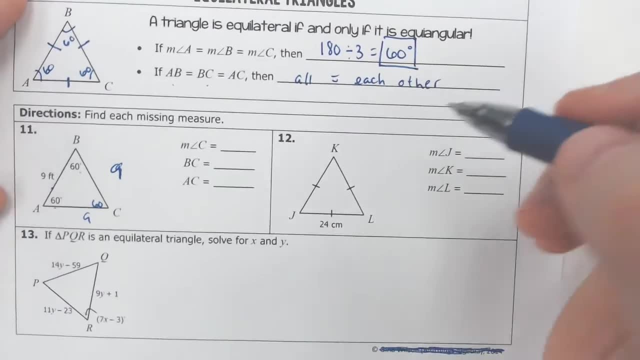 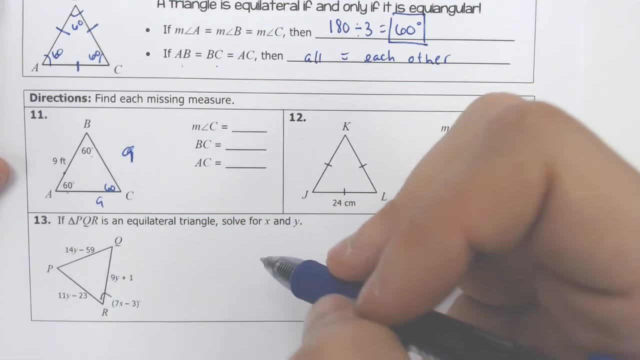 So all the sides are 9, all the angles are 60, and if that is the case, then normally you will be just setting things equal to each other. so in this case, on number 13, I need to solve for X and I need to solve for Y. I am going to start the. 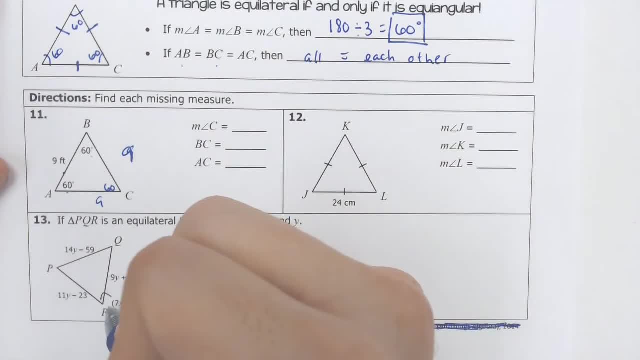 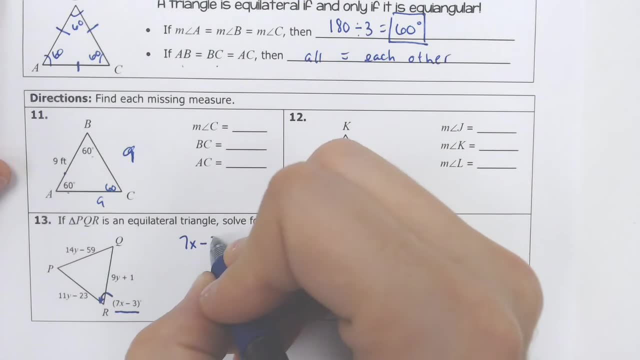 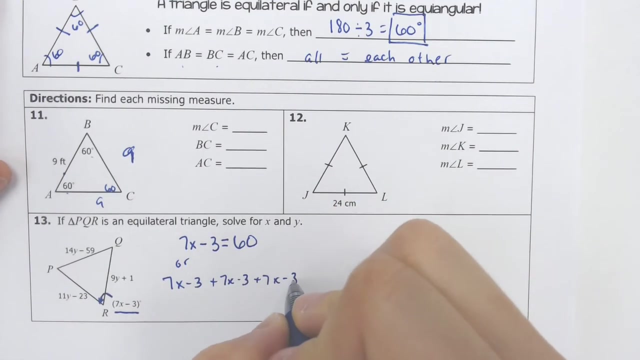 problem and I'm going to encourage you to finish it. so if this X part represents the angle of an equilateral triangle, all angles of an equilateral triangle have to equal 60. the other option would be to do 7 X minus 3 plus 7 X minus 3 plus another 7 X minus 3 to equal 180. that would be the longer. 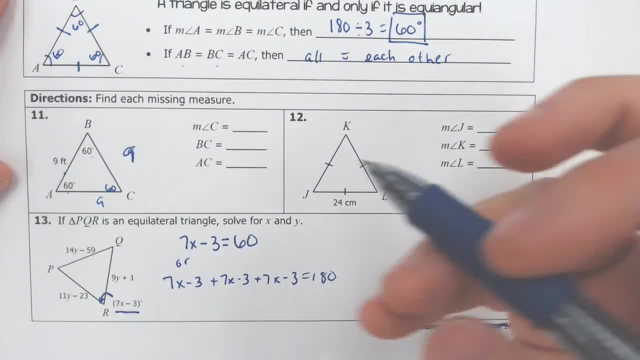 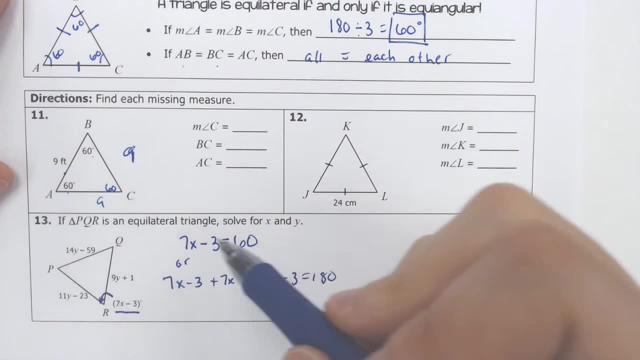 option. I would not recommend that for the Y's. we're going to be solving for the side. so all three of these sides are equal. that means you could set any of them equal to X, any of them. So pick whatever two you like, whichever two you like, and set them equal to. 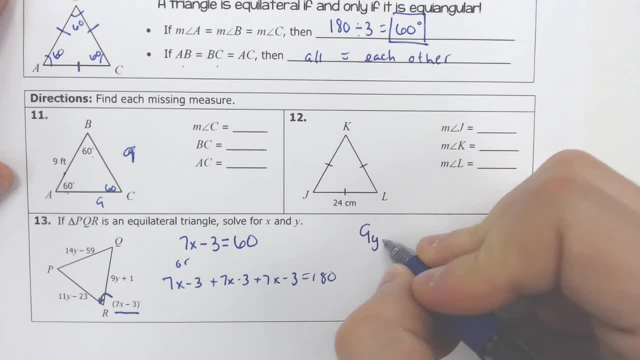 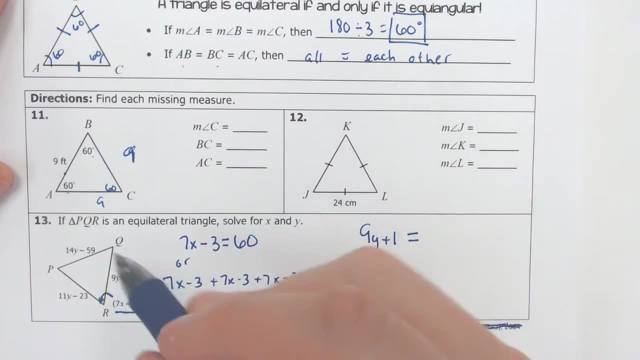 each other. So I know that most of you would like 9y plus 1.. So you just need to set it equal to whatever other equation, whether that be the 14y minus 59 or the 11y minus 23,. you need to set it.